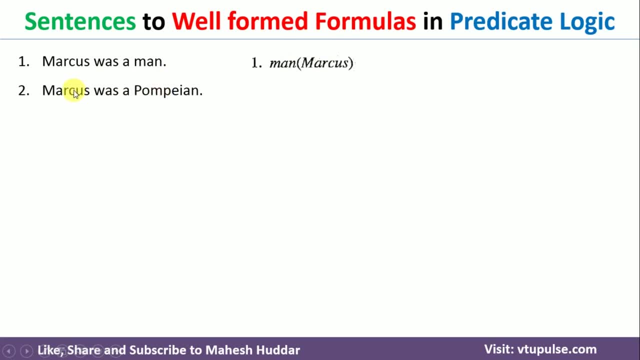 The same thing here. Pompeian is one class here. Within that, Marcus is one entity again. So, that's the reason you can write something like this, Pompeian, Marcus over here. Now, coming back to the third fact, all Pompeian were Romans. So, in this case, we have been given all Pompeians. All Pompeians in the sense, like, we need to consider for all x over here. So, that is the one thing and if x is a Pompeian, then that particular x is a roman here so that is what the meaning of this particular sentence or a fact so that can be written something like this for all x because all is there we have to take for all x and if x is pompeian that is what i have written here if x is a pompeian then x is a roman over here is now coming back to the fourth one caesar was a ruler again in this particular case ruler is one class within that particular class caesar is one entity so that's the reason you can say that ruler of caesar in this case again it is a quite simple fact or a sentence in this case so that can be converted into predicate logic very easily consider the next example that is all romans were either loyal to caesar or hated him so because we have again all here the very first thing what we need to do is we need to take for all x and we need to consider roman x that is if x is a roman then they are either loyal to caesar or hated him 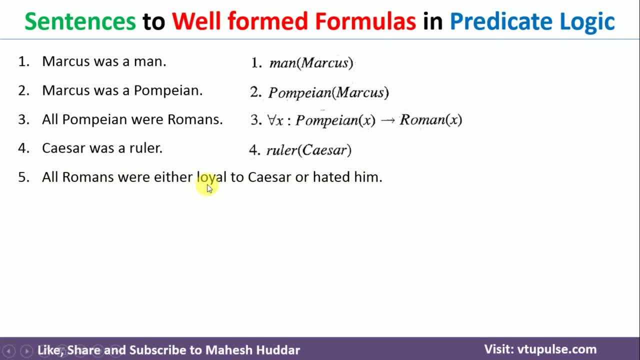 so we have to take two classes again here one is loyal to another one is hate the loyal to will take two parameters that is x loyal to caesar or hate will take again two parameter that is hate x comma caesar again here so this can be written something like this one for all x if x is a roman then x is loyal to caesar that is the one possibility or x hates this particular person over here so either of these particular possibilities will exist here either x is loyal to caesar or x is hate this particular caesar in this case so there are two things we can achieve if x is a roman in this particular case coming back to the next fact that is everyone is loyal to someone again because we have loyal to here loyal to will take two parameters that is x is loyal to caesar similar to that one if i take x comma y x is loyal to x is equal to x is equal to x over here that's the to y in that case okay so now if you look at this particular thing everyone is loyal to someone so if i say the quantity of this particular x and y x is everyone and second parameter that is y is someone here so that's the reason we will write for all x there exist y loyal to x comma y that is nothing but x is loyal to y that is for sure but what is the quantity of this particular x is this is for all x because everyone everyone is written here and similar to y y is someone here that's the reason we have written there exist that is this x is loyal to one or more persons 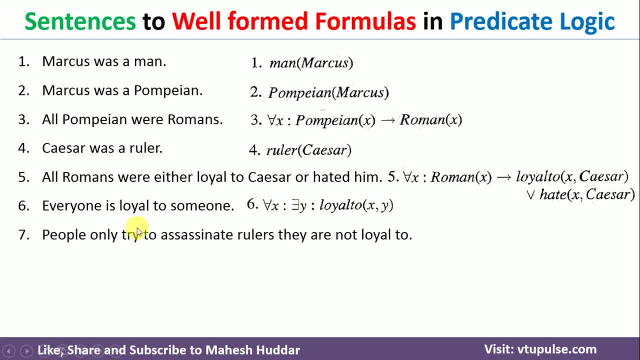 over here that is what we can say in this case coming back to the next fact that is people only try to assassinate rulers they are not loyal to that is a case we have to check whether the particular person is people and then this particular people will try to assassinate rulers they are not loyal to that is a case we have to check whether the to assassinate rulers here. So, if x is a people, we cannot take people here, I will take person, that's the best option. If x is a person and y is a ruler, that x will try to assassinate y if they are not loyal to one another. The meaning of this one is for all x, for all y, if x is a person and y is a ruler, if x is a person and y is a ruler, try to assassinate, that is x will try to assassinate y, that is what I have written here. 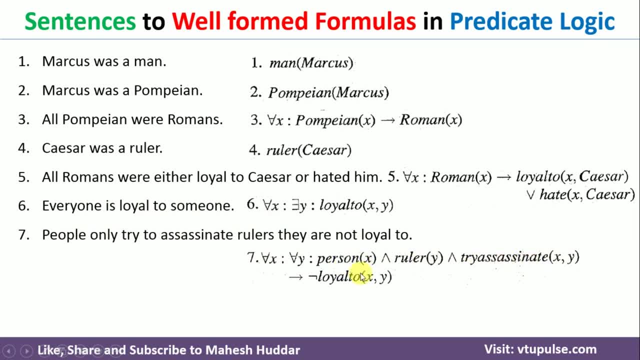 If all these conditions are satisfied, then x is not loyal to y here, because if x is loyal to y, this will not happen. If x is a person and y is a ruler, x will try to assassinate y, the meaning of this one is x is not, loyal to y over here. So, that's the reason we have taken negation of this particular statement 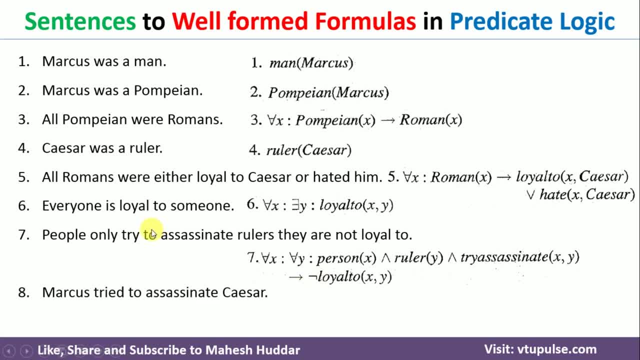 here. Now, coming back to the eighth fact here, that is Marcus tried to assassinate Caesar in this case. So, it's a very simple statement here, Marcus tried to assassinate Caesar. What is the meaning of this particular predicate statement? Try to assassinate x comma y, that is x is trying to assassinate y over here. In this case, x is given as Marcus and y is given as Caesar, so Marcus tried to assassinate Caesar in this case. So, that is how actually you can write this particular statement over here. Now, coming back to the last one, that is all men are people. 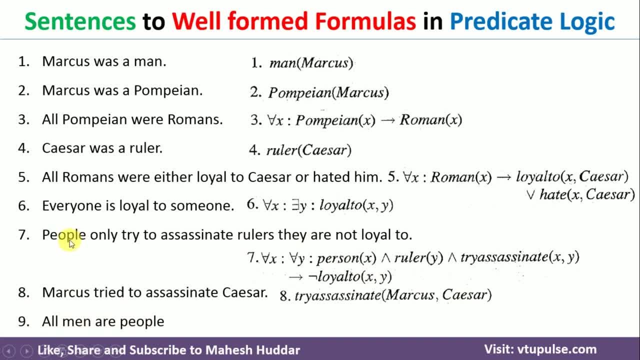 Again, people I have already told you, rather than taking people, you can take person x over here, 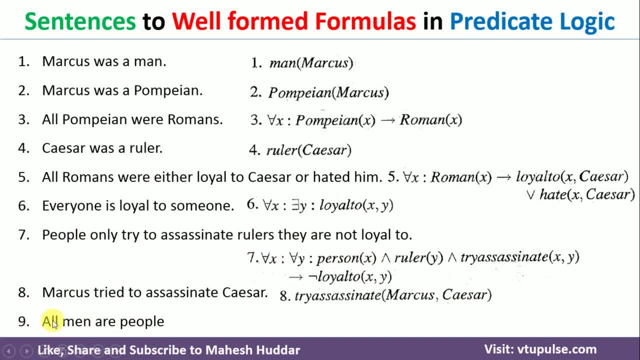 because all is there, we have to take for all x. If x is a man, then x is a person here. So, that is a very simple statement we can write. For all x, if x is a man, then x is a, 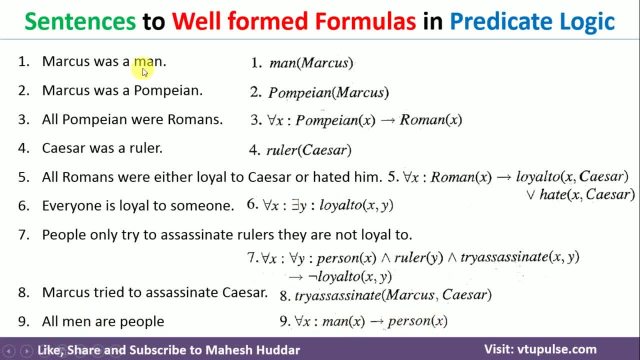 person over here. So, this is how actually we can convert facts or sentences into well-formed formulas in predicate logic. In this video, I have explained only the conversion part. In the next 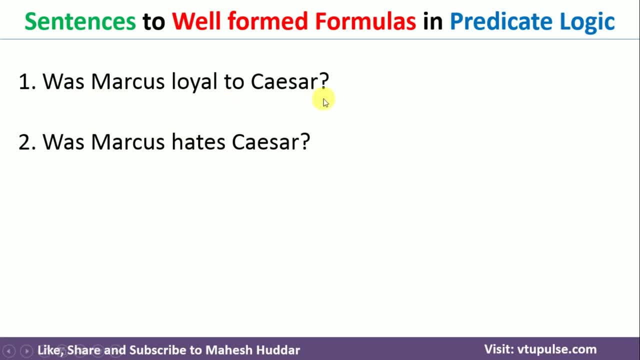 video, we will discuss how can we prove some of these particular inferences, like was Marcus loyal to Caesar? In this case, we need to check whether Marcus was loyal to Caesar or not. And similarly, 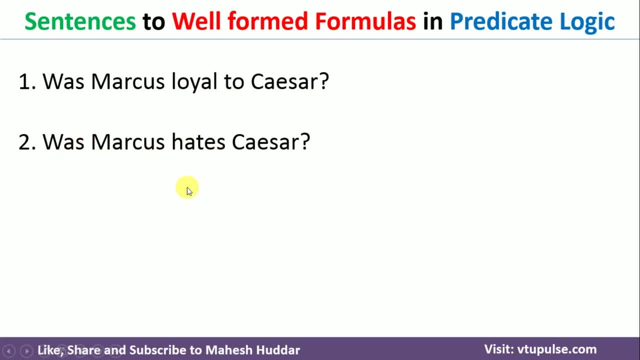 we have one more example here, was Marcus hates Caesar? So, 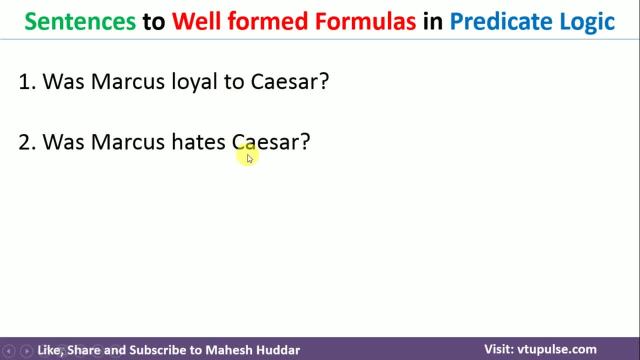 I have already solved these particular inferences also. The link for that video is given in the description below. You just follow that particular video to understand how can we prove such kind of 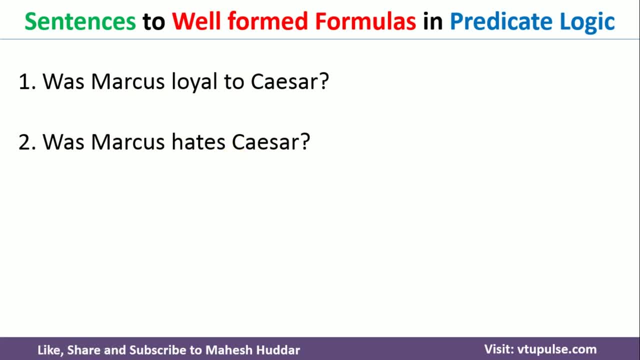 statements with the help of predicate logic in this case. I hope the concept is clear. If you like the video, do like and share with your friends. Press the subscribe button for more 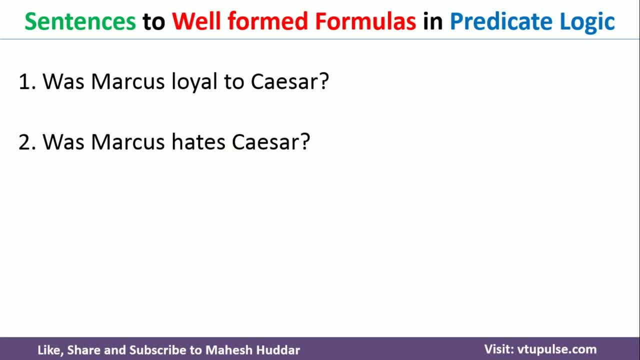 videos. Press the bell icon for regular updates. Thank you for watching.